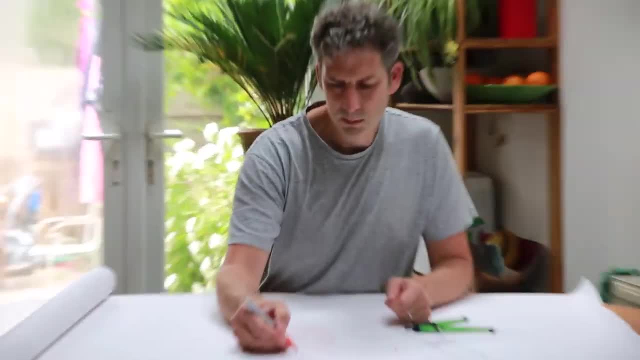 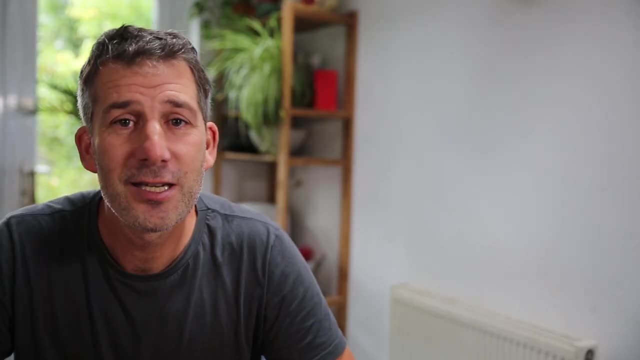 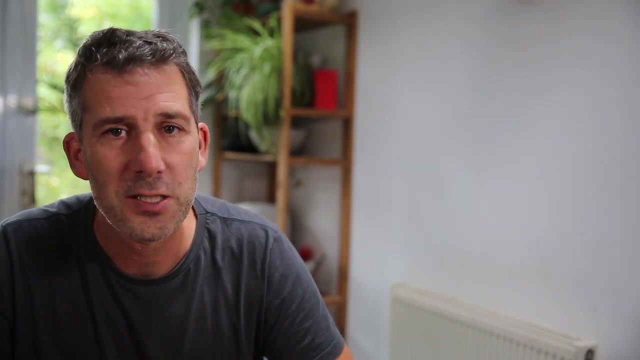 to help to explain how we do that. So percentage is one of those things that we do in maths that actually they come up in real life all the time, So it's a concept that's well worth practicing and mastering. In this video, we're going to look at some nice, simple 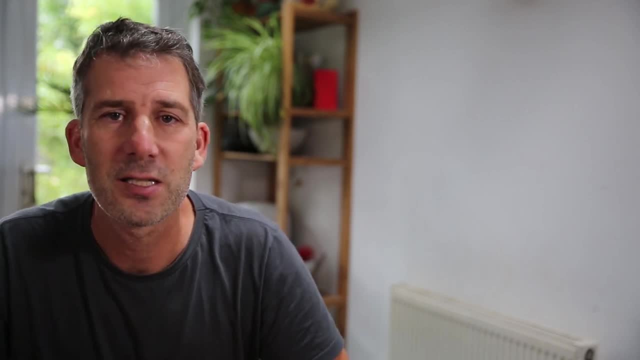 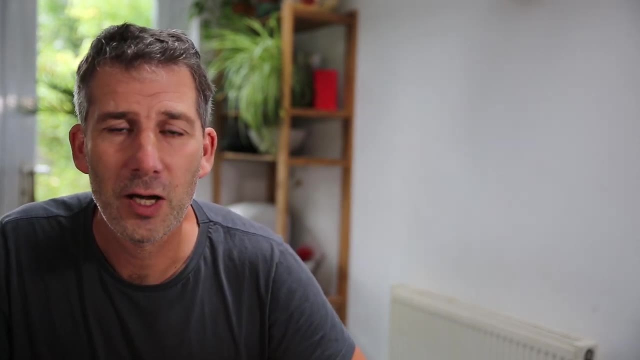 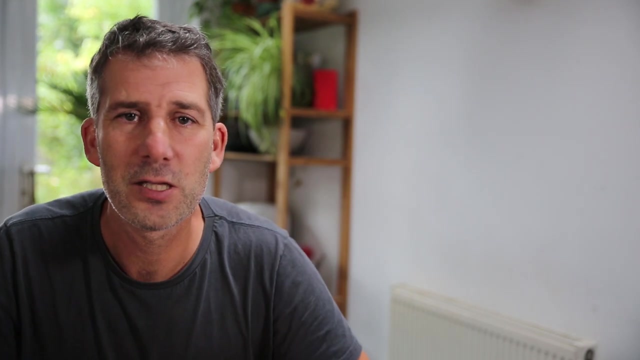 methods to calculate percentages, and then I'm going to do a second part as well, where we'll look at some more advanced methods. So what are percentages all about? Well, percent means out of a hundred. So if you're finding 1% of something, it just means you're splitting something up into. 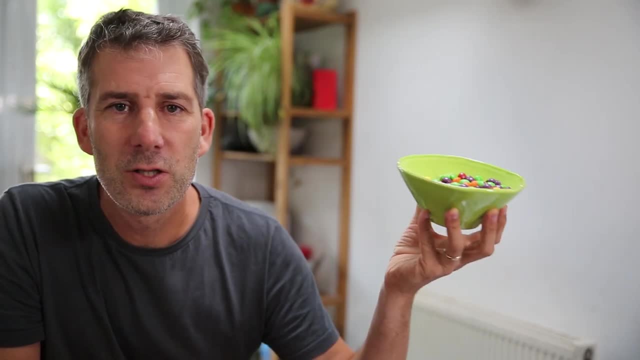 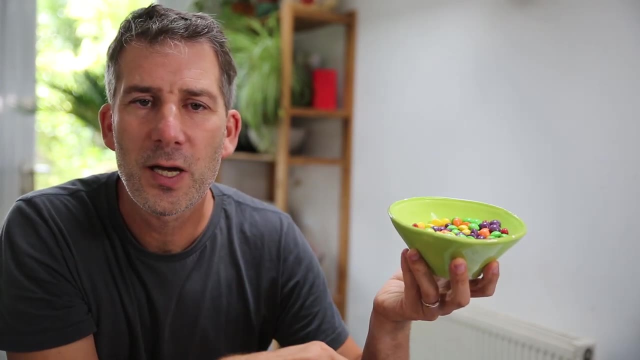 a hundred equal parts. If I take these 200 sweets and I divide them up into a hundred equal piles, then each of those piles will represent 1% of the total amount, In other words, 1% of 200.. So let's do that now. 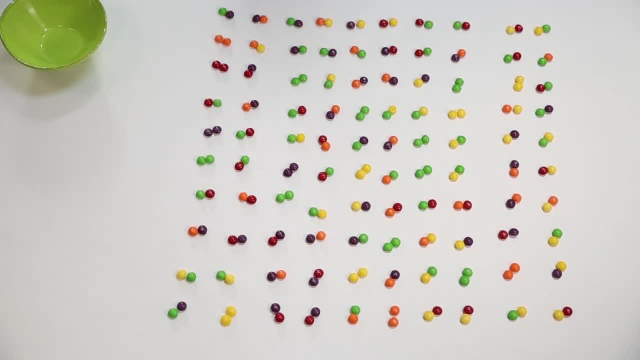 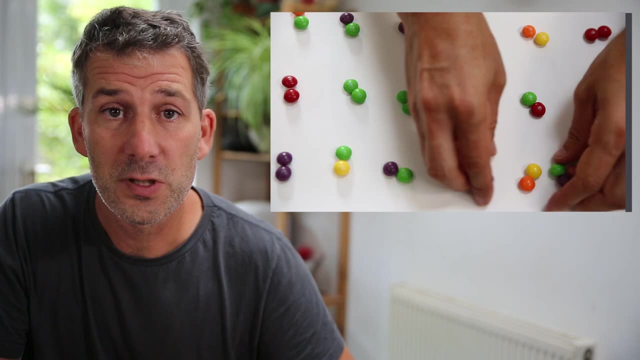 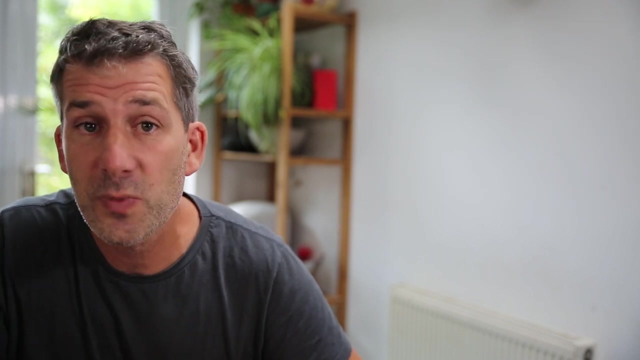 You can see that there are two sweets in each group, so 1% of 200 is 2.. And if you wanted to find 3% of 200, you just put three of those groups together. That makes six sweets, so 3% of 200 is 6.. If you wanted to find, say, 17% of 200, you 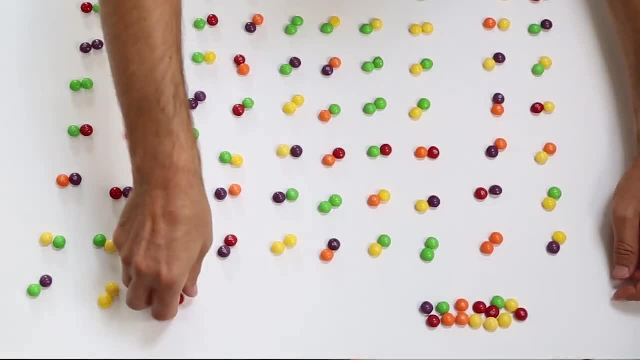 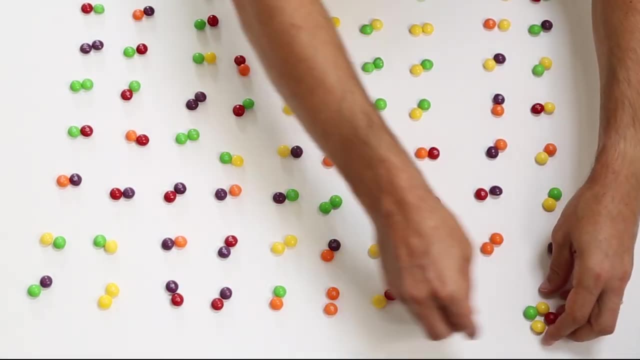 just need to put 17 of those groups together, count up how many sweets you've got. So 17% of 200 is 34.. But you're not always going to have hundreds of skittles with you, So let me quickly show you how you do it without Let's say I want to. 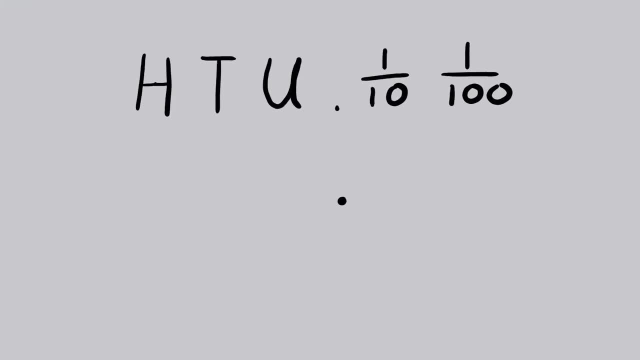 find 6% of 700.. I start by finding 1% of 700.. So I do that by dividing by 100.. That gives me 7.. And then to find 6%, I just multiply that by 6.. So I do 7. 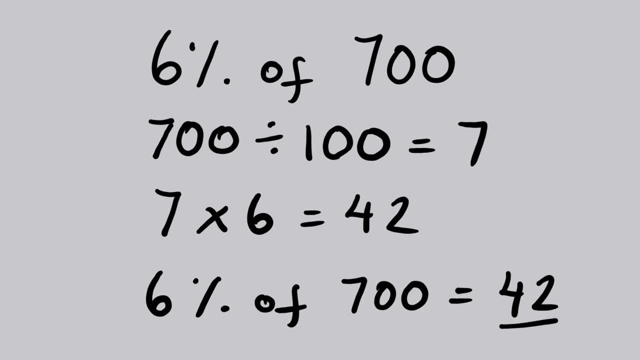 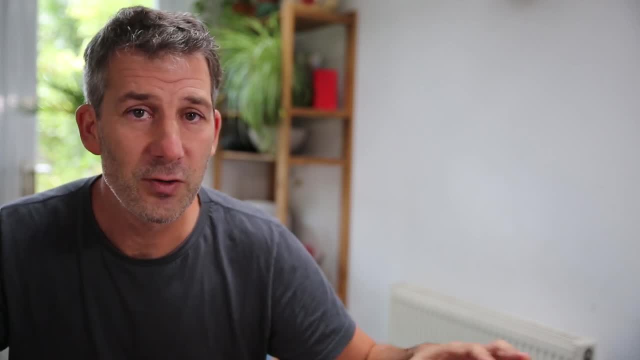 times 6, which is 42. So 6% of 700 is 42. Now that's a perfectly good method. You could pretty much find any percentage of any amount using that method, Splitting it up into a hundred and then add as many groups together as you want. 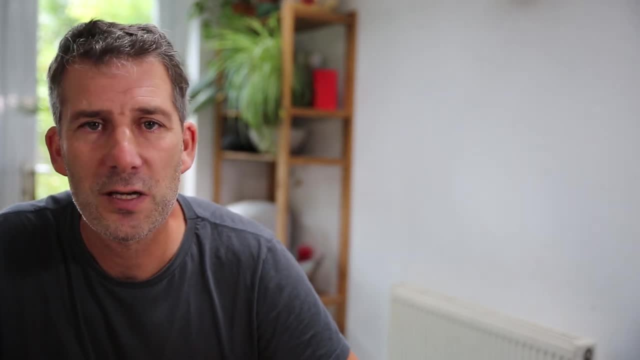 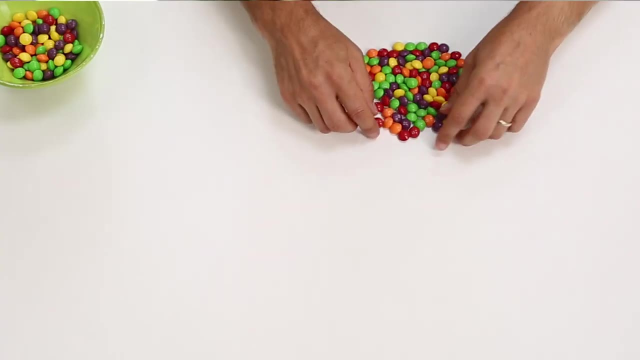 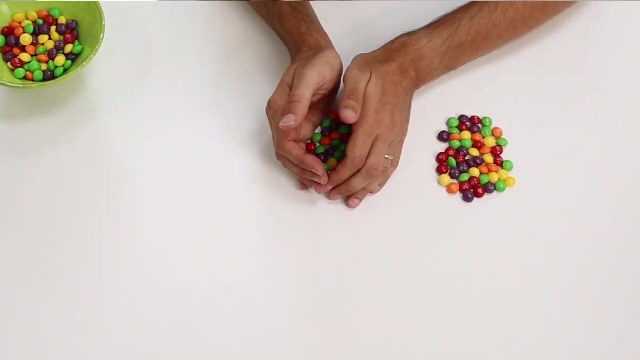 But it's not always the easiest or the fastest method, So we're going to look at some different techniques that will be a little bit easier and a little bit faster for lots of situations. Now I've got a hundred sweets here, So each sweet represents 1%. If I split those into two groups, I got 50 sweets in each. 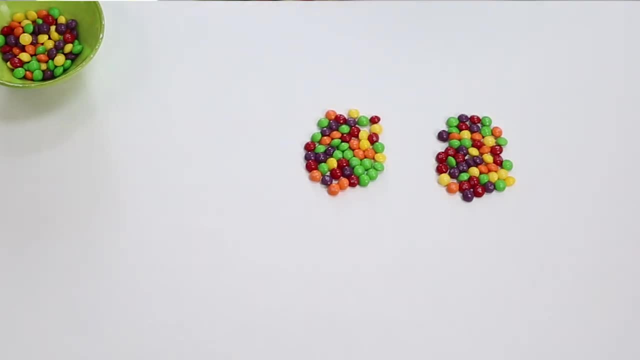 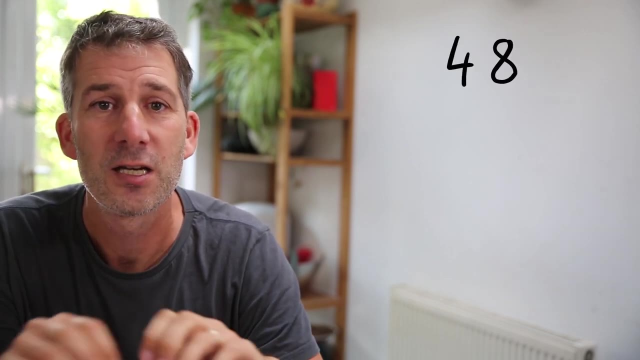 group. In other words, I've got 50% in each group. Okay, so to find 50% of something, you just divide it by 2.. You halve it. Alright. so 50% of 48, just divide that by 2.. 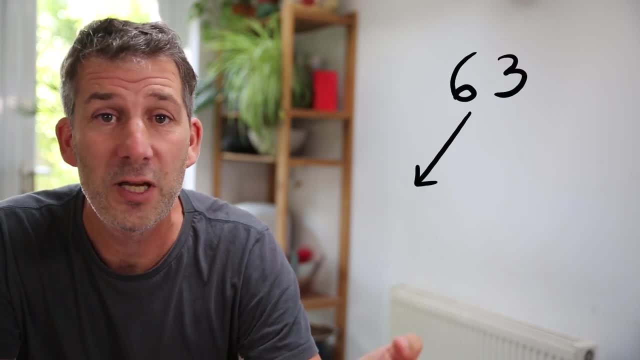 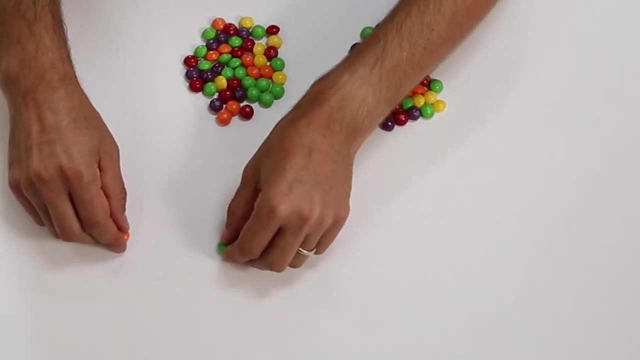 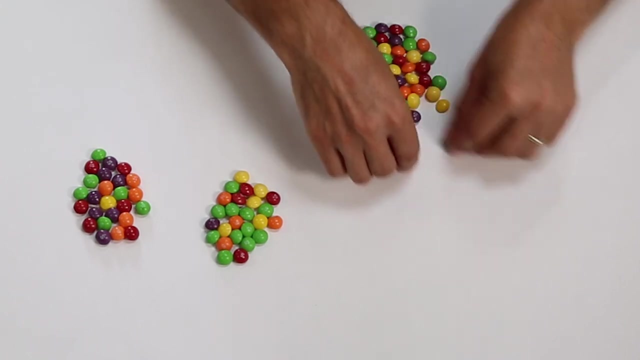 So it's 24.. 50% of 63 is 31 and a half, Just divided it into two. Now, moving on from that, if I then split each of those groups up into two, I've got four groups overall. In other words, I've split my hundred sweets up into four groups And 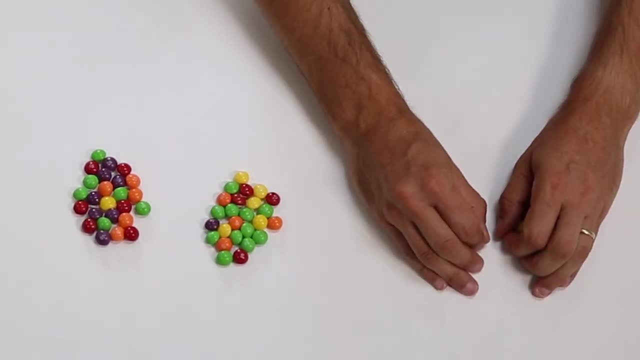 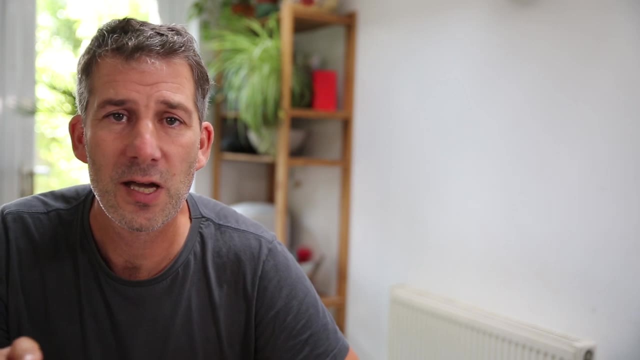 I'll have 25 sweets in each group. So if you divide something by four, you found 25% of it, And an easy way to do that is to halve and then halve again. Okay, so to find 25% of something, you halve it and 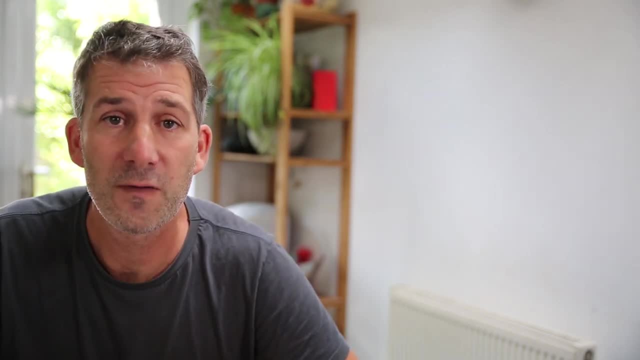 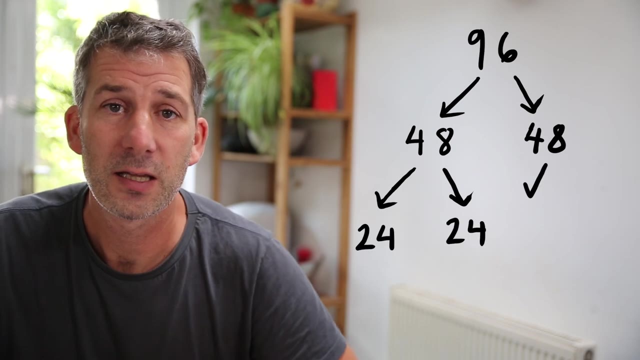 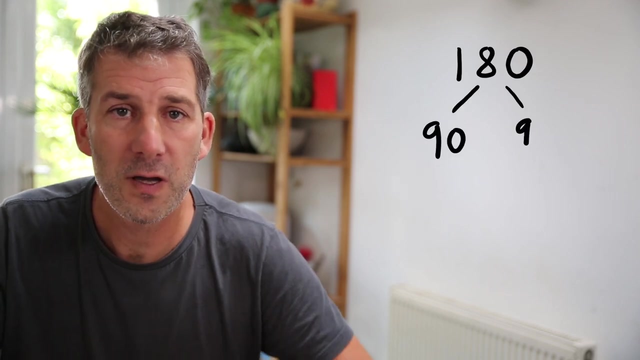 then you halve it again. For example, 25% of 96. I could halve it to find 48. Then halve it again, that would be 24.. 25% of 180 and halve it, which would give me 90. 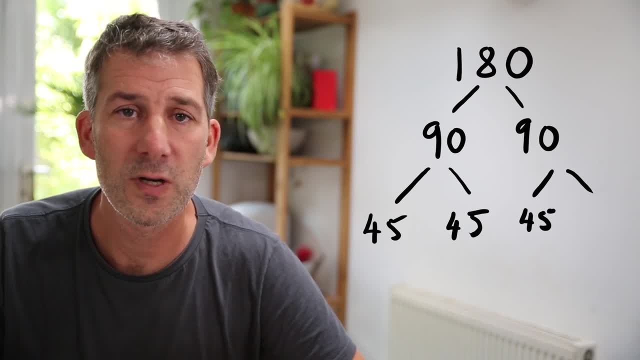 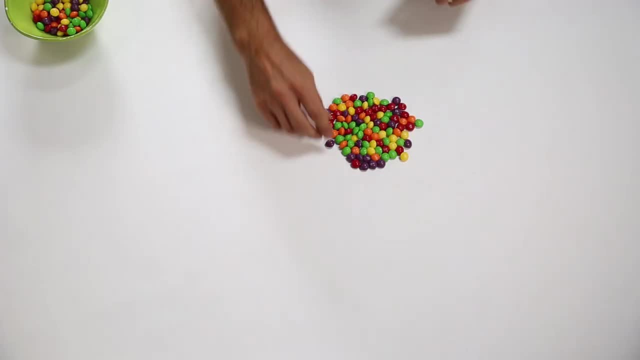 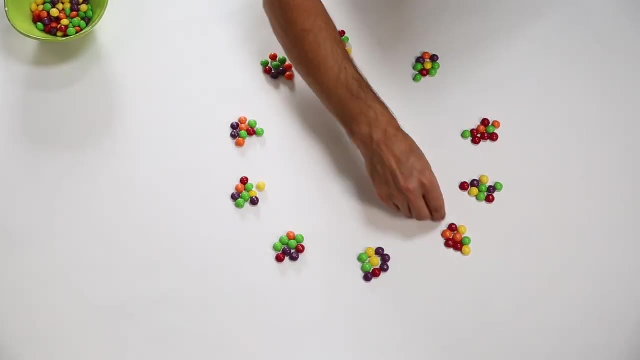 and then halve it again, which would give me 45.. So 25% of 180.. would be 45, okay? so that's how you find 25 or something. back to our 100 sweets. then if i split the 100 sweets up into 10 groups, i've got 10 sweets in each group. so if you divide something, 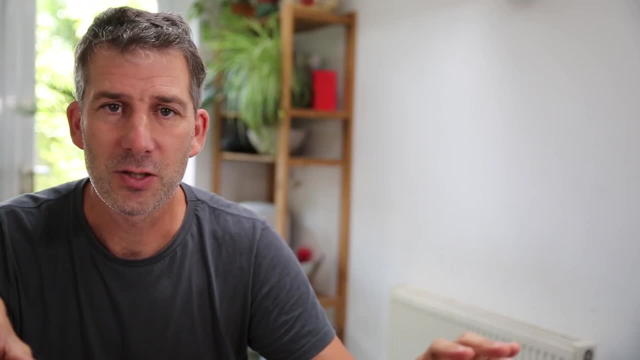 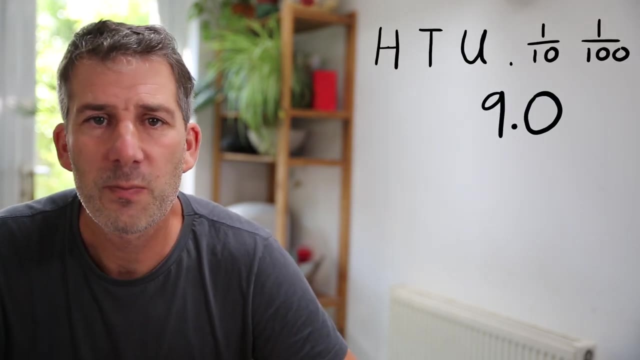 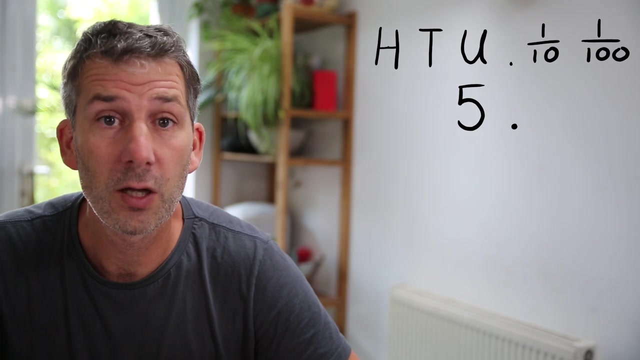 by 10, you end up with 10 in each group. okay, so to find 10 of something, you divide by 10. so 10 of 90 would be 9, 10 of 150 would be 15, 10 of 5 would be 0.5. okay, you just divide by 10. 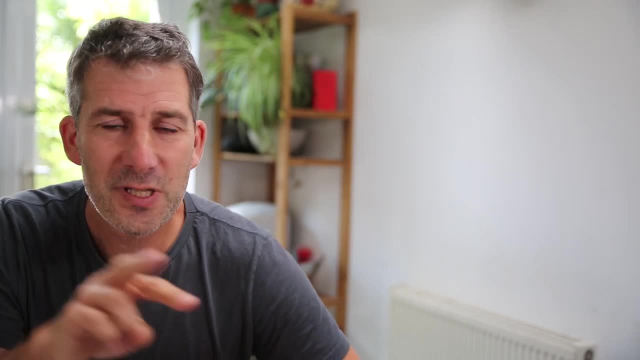 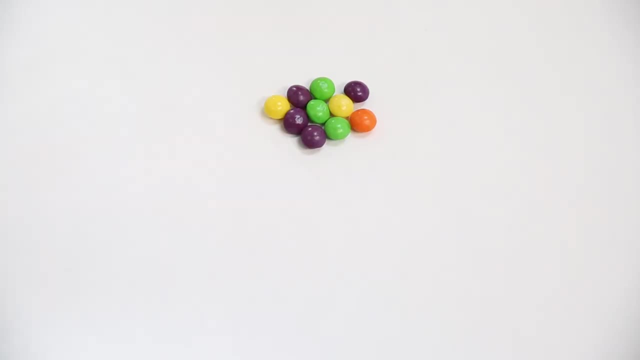 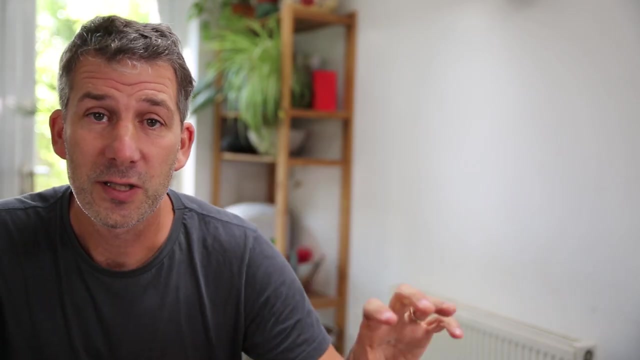 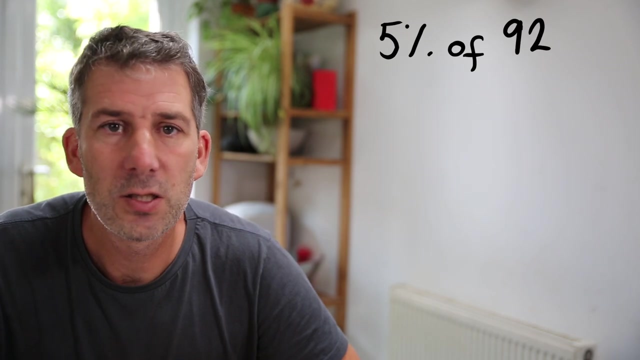 following on from that, there are other percentages we can work out from that. so if you've divided something by 10 to find 10, if you split each of those groups up into two, you've got five percent. okay. so to find five percent, you divide by 10 and then half it: okay. so five percent of uh 92- okay, i find 10. 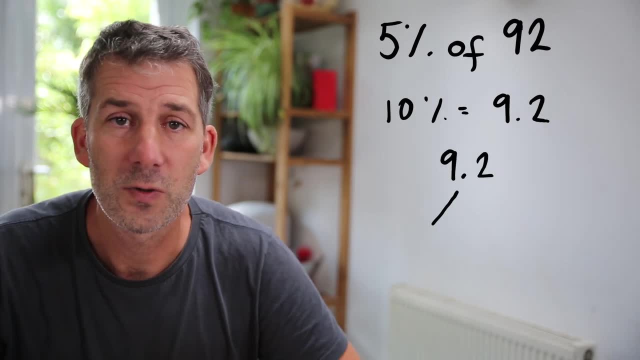 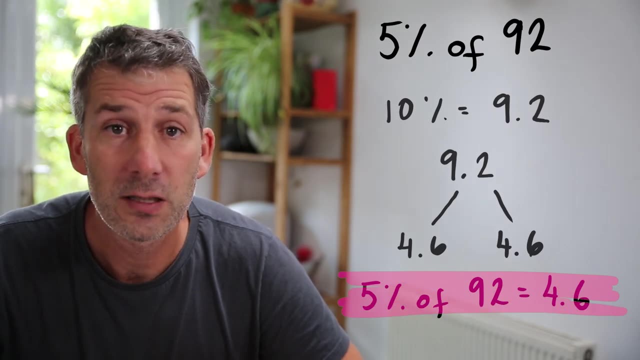 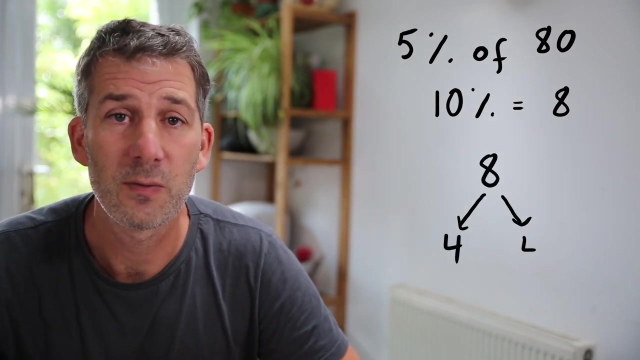 which is 9.2, and then half of that which is 4.6. so 5 of 92 is 4.6, 5 of 80. i divide by 10 to give me 10, so that's eight, and then divide by two and that will give. 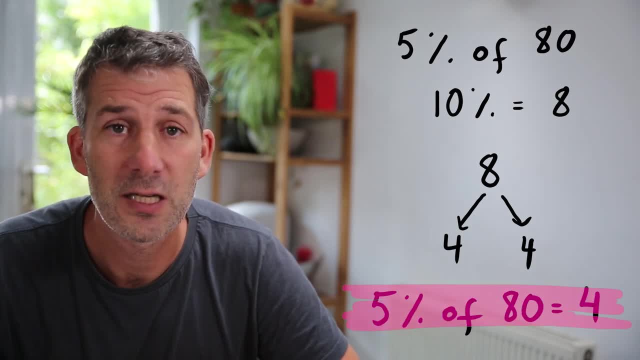 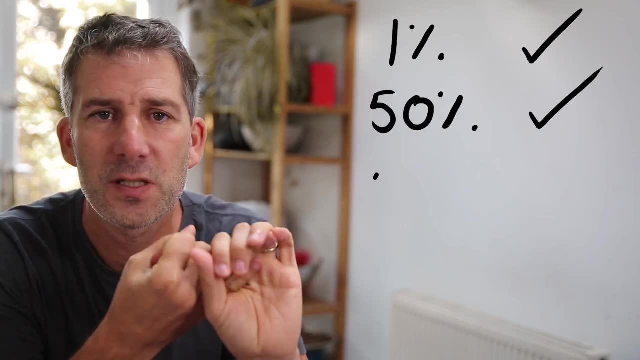 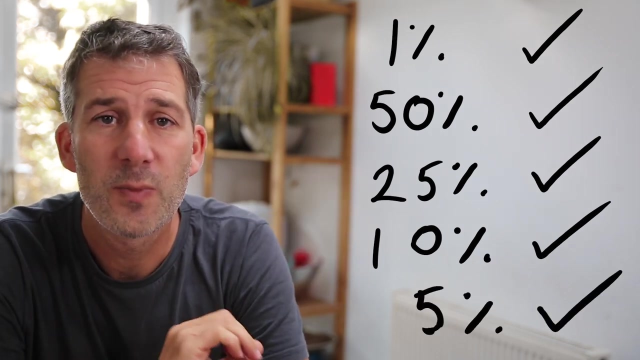 me five percent, which is four. okay. so five percent of eighty is four, all right. so let's recap. we know how to find one percent of something. we know how to find fifty percent of something, twenty five percent, ten percent and five percent. we can now combine those to be able to find any percentage of anything. 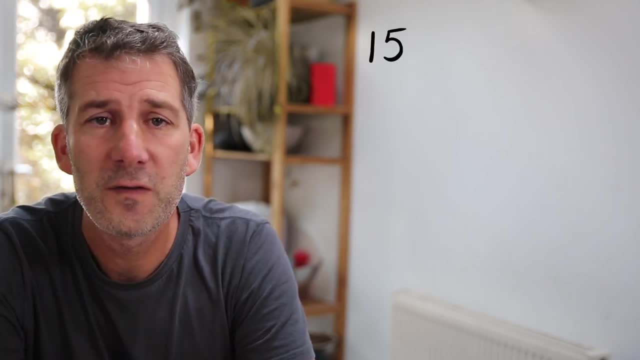 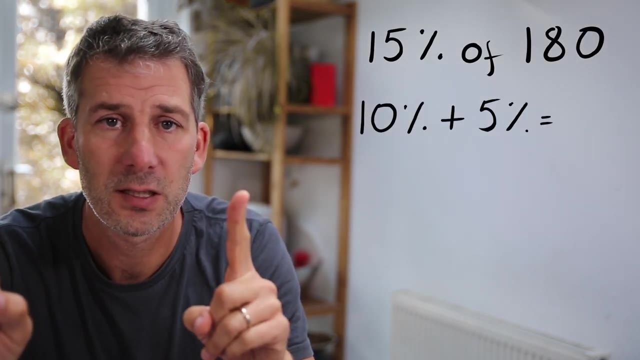 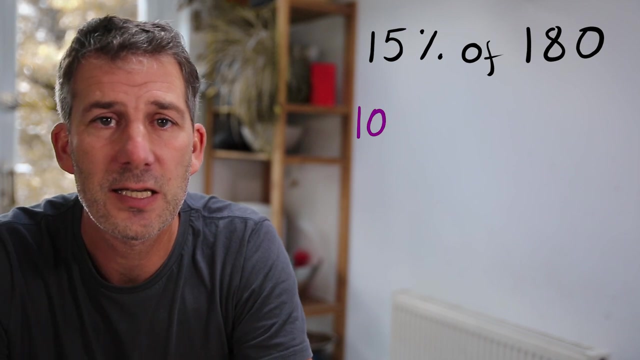 really so. let's say we wanted to find fifteen percent of a hundred and eighty. what i'm going to do is i'm going to find ten percent and then five percent and add them together, because ten percent and five percent is fifteen percent. so ten percent of 180 is 18, and then five percent is half of that, which is nine. okay, so ten percent. 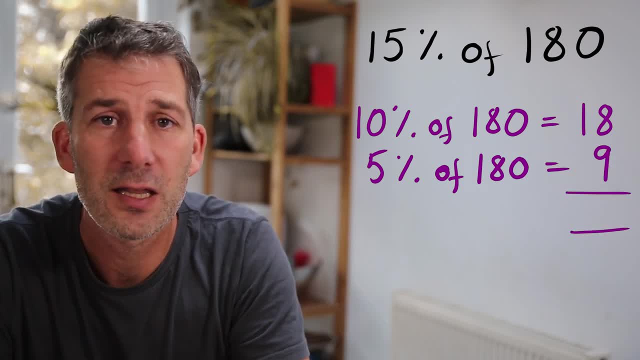 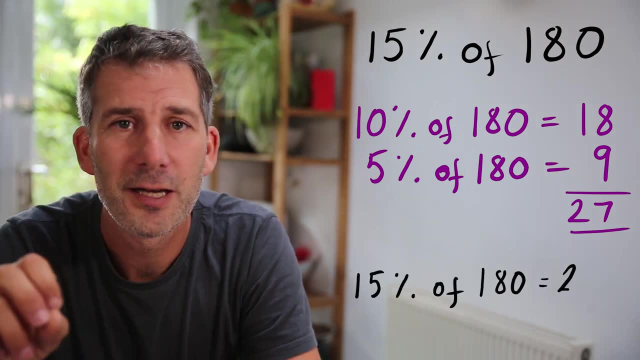 is eighteen. five percent is nine. if i add those together, which is 27, i've got 15. so 15 of 180 is 27.. let's say we want to find 15 of 140.. pause the video. have a go on your own. 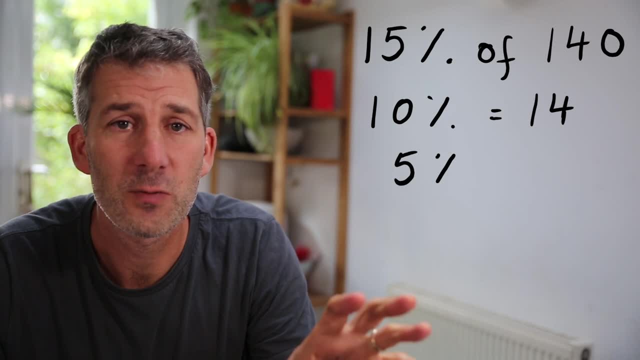 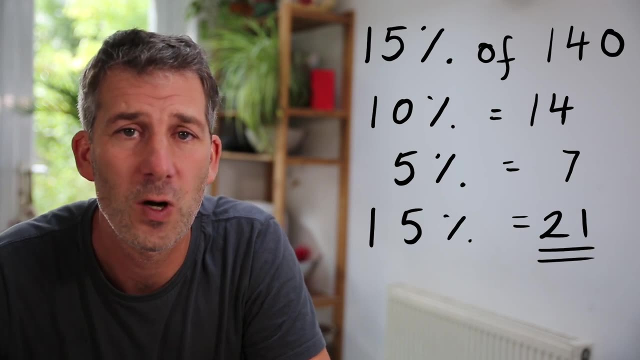 i'll find 10, which is 14, and then 5, which is 7. just add those together. so 14 add 7 is 21.. the 15 of 140 is 21.. so those i chose nice easy numbers there, but the principle is the same even. 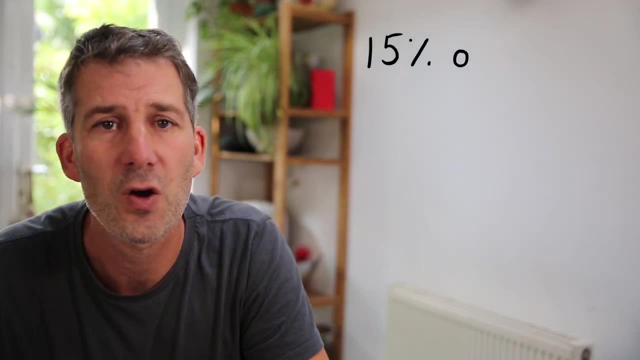 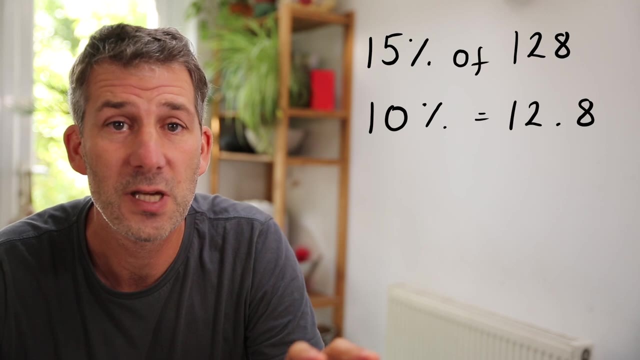 if the numbers aren't quite as nice. so let's say i want to find 15 of 128. i would still just find 10, which would be 12.8, and then five percent, which would be 6.4, and i'm going to add those two. 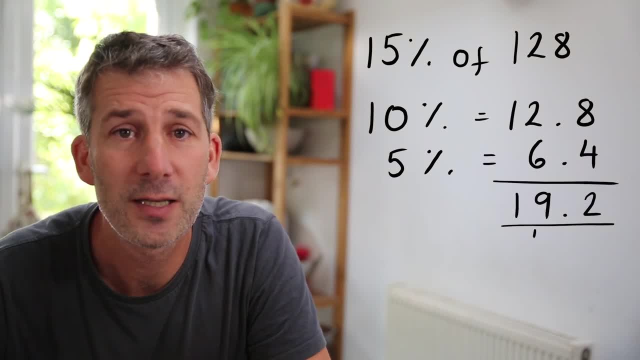 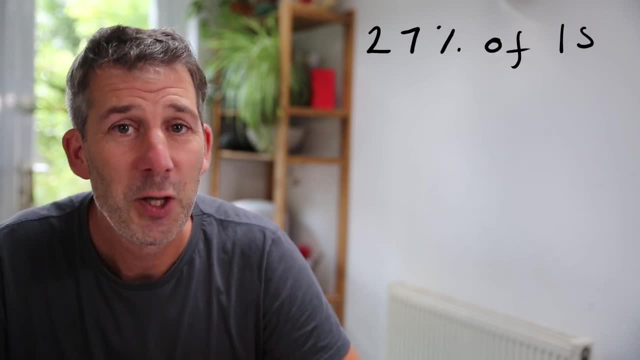 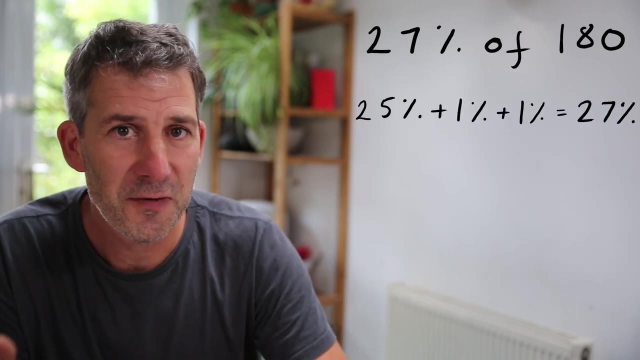 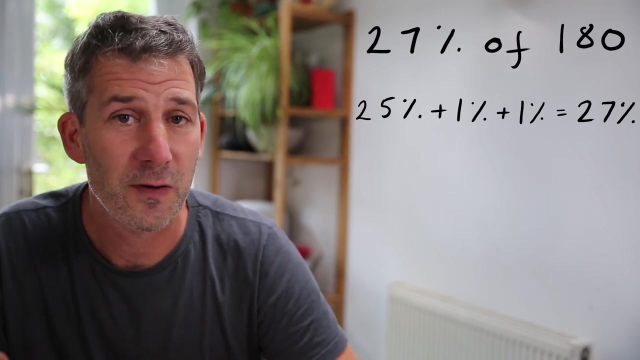 together, which would give me 19.2. if you want to find 27 of something- let's say we're doing 27 of 180- then you can find 25 and then add on one percent, then add on another one percent, because 25, add one percent, add one percent is 27 and we know how to find those. we know how to find 25. 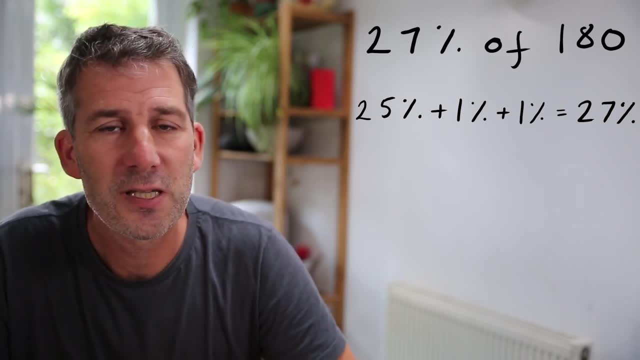 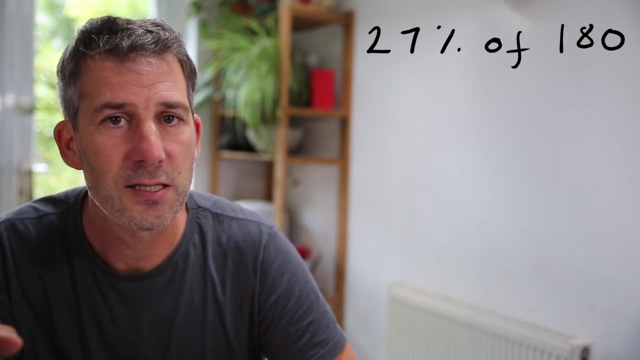 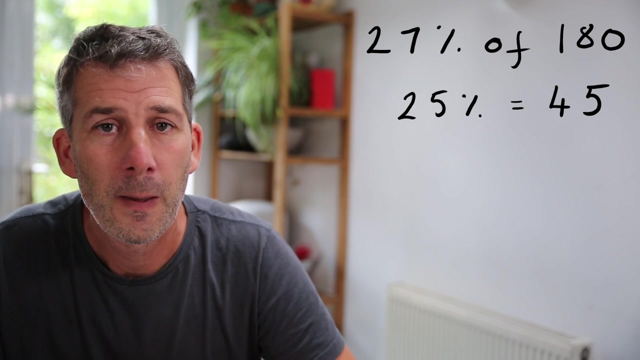 we know how to find one percent. okay. so 25 percent of 180. you remember we halve it and then halve it again. so half of 180 is 90, half that you've got 45. so 25 is 45. i'm just going to make a mental note of that. one percent, you'll remember we divide by 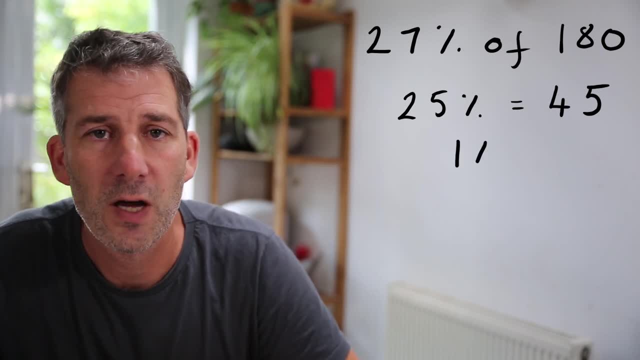 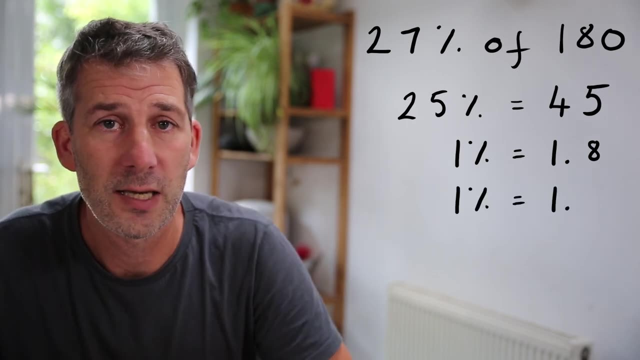 a hundred to find one percent of something. so one percent of 180 is 1.8, but i actually want two of those, so i want 1.8 and 1.8 and that's 3.6. so we've got the 25. 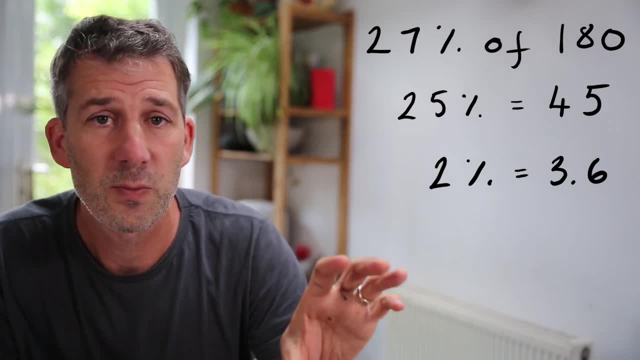 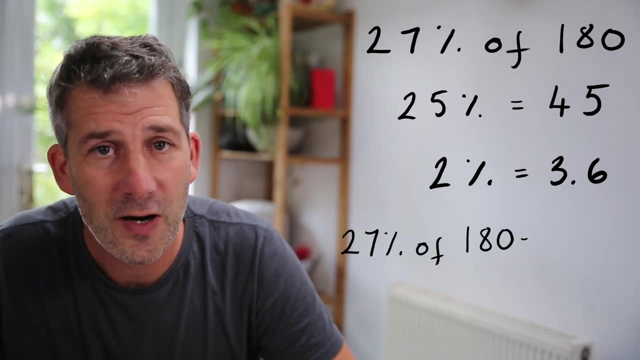 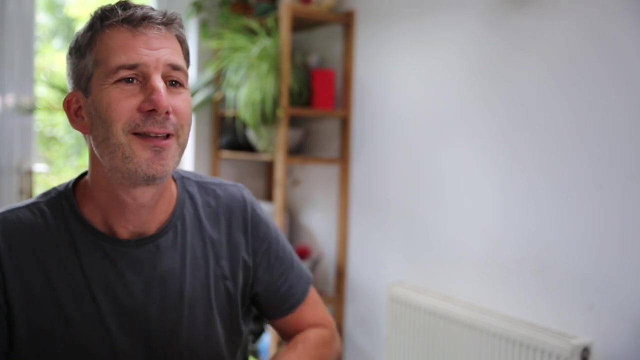 which is 45, and we've got the two percent, which is 3.6. we add those together, we've got 48.6. okay, so 27 of 180 is 48.6, okay, okay, okay. what about 38 of 127? 38 of 127? yeah, okay, all right, so those. 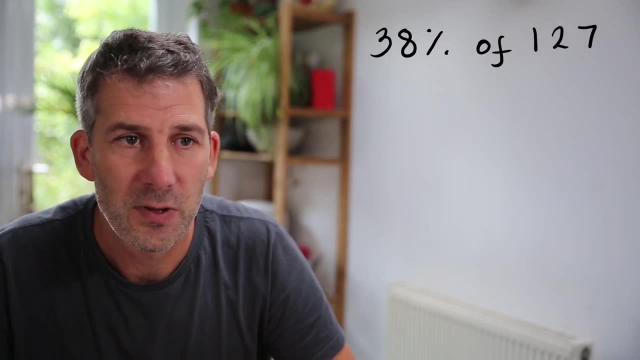 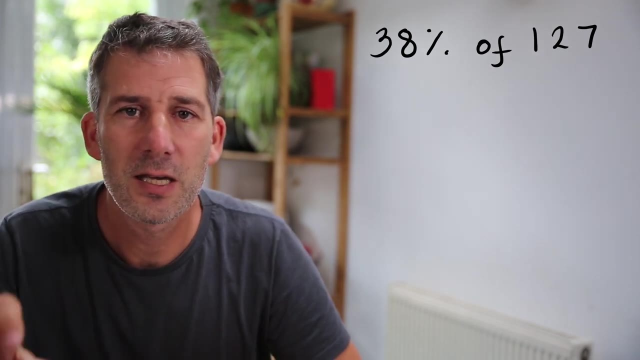 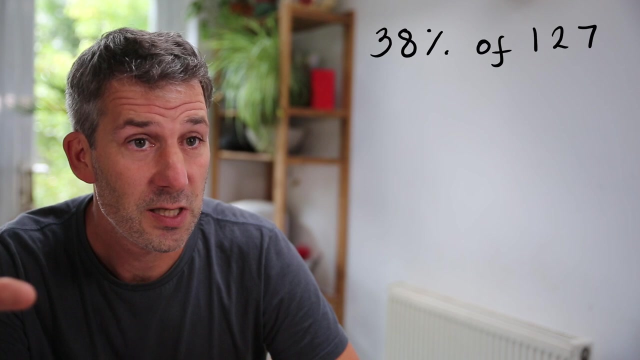 numbers are a bit more awkward, but we can do the exact same thing. so what was it? 20, 38, 38, okay, so 38 i can make. actually, there's lots of different ways that i could make 38, but i'm going to go with. i could find 25, and then, if i added on 10, i'm up to 35. 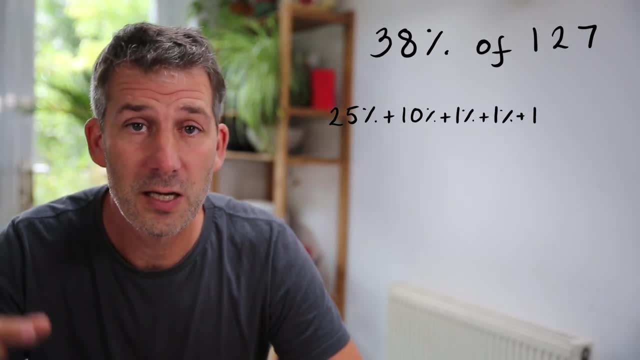 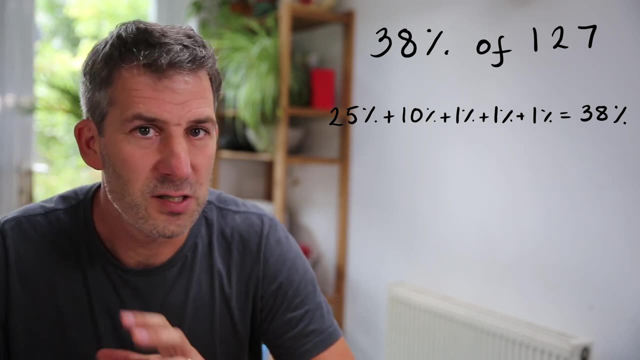 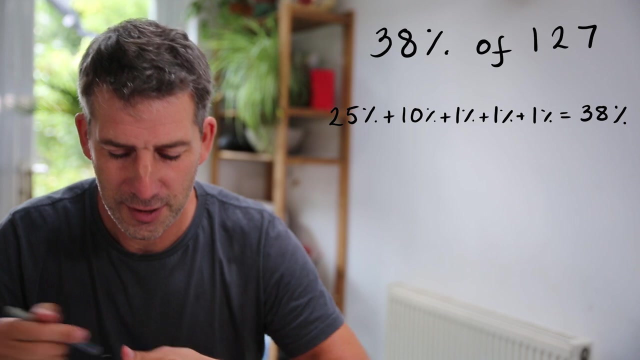 and then you can add on three ones. okay, so you can make 38 by doing 25 add 10, add one, add one, add one. okay, um, because those are all percentages that we know how to calculate easily. all right, so i've already forgot what the number was. what was it? write it down, thank you. so 38. 38 of 127 of 127. 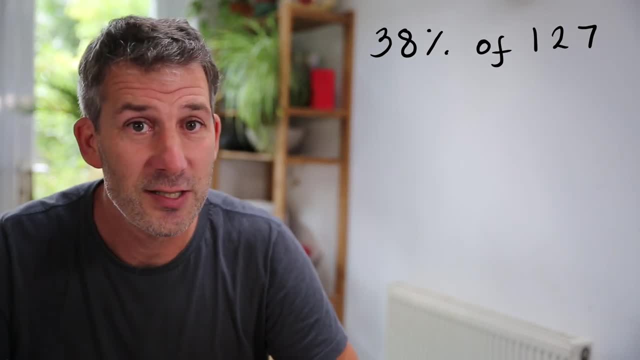 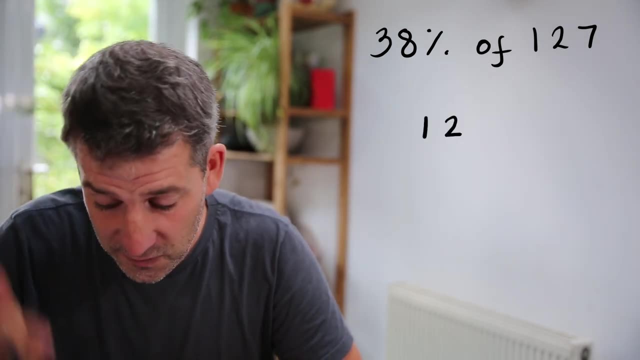 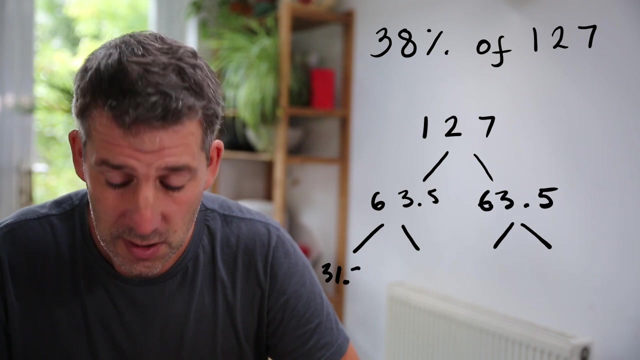 so this is definitely going to be one of those ones where i'm going to have to actually write stuff down as opposed to making a mental note. okay, so 25 of 127. well, if i have it, that gives me 63 and a half 63.5, and then half of that is 31.75. 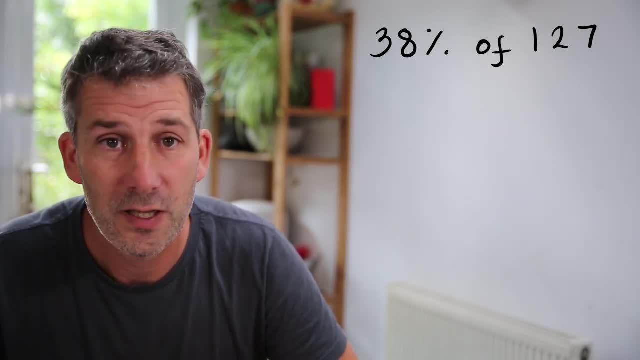 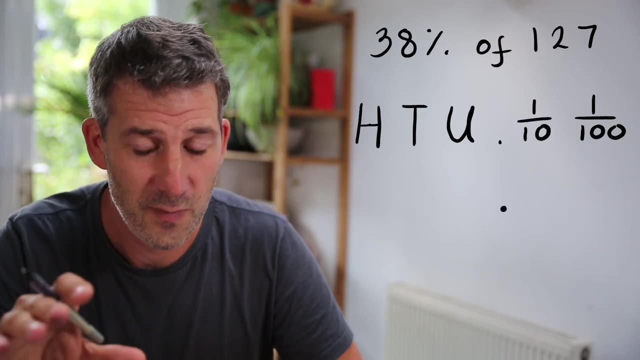 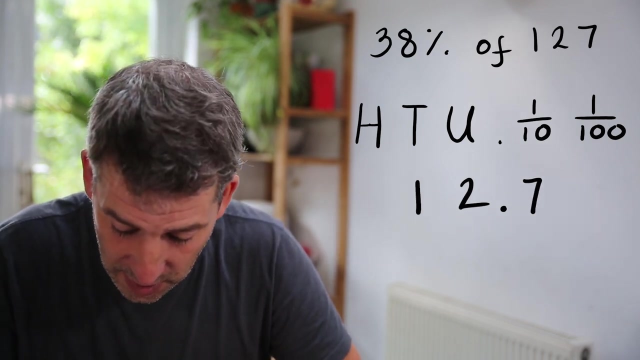 so 25 of 127 is 31.75. to find 10, i divide it by 10, right, you remember that one. to find 10, you divide it by 10.. so 10 of 127 is 12.7, making out of that 12.7. um, so i've got 25, i've got 10. 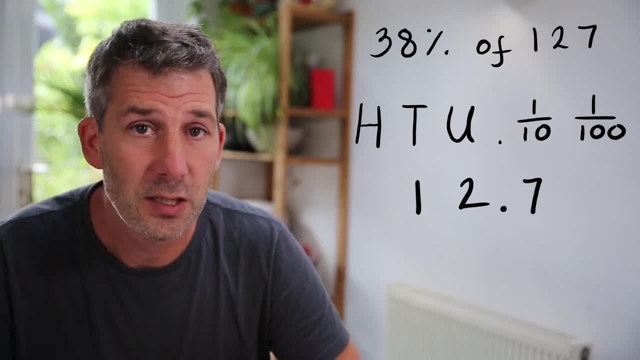 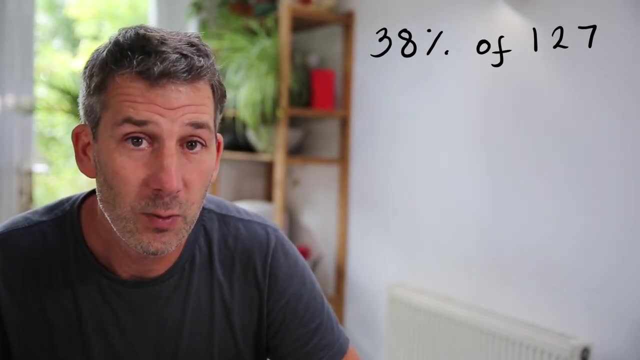 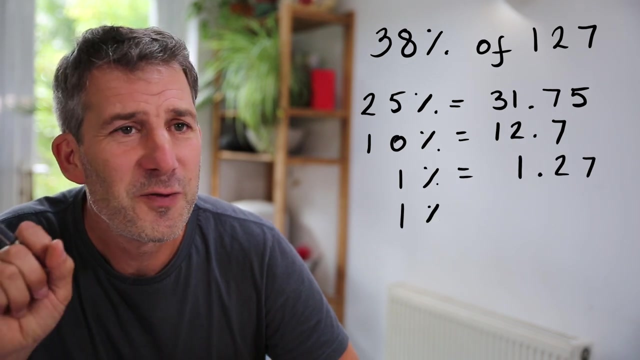 now i need by three, one percent, okay. so one percent you divide by a hundred, so that'll be 1.27. so i'm going to write that down. so 1.27 add 1.27, add 1.27. so you've chosen some nice awkward numbers for us, which. 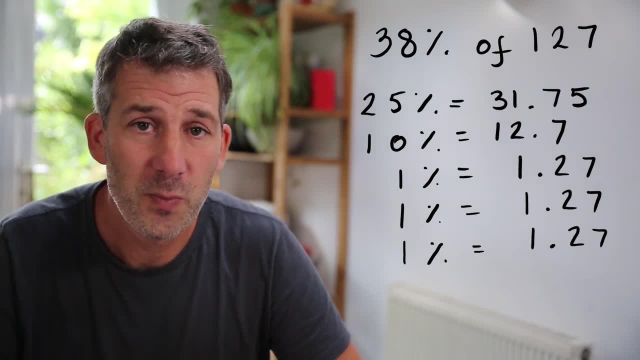 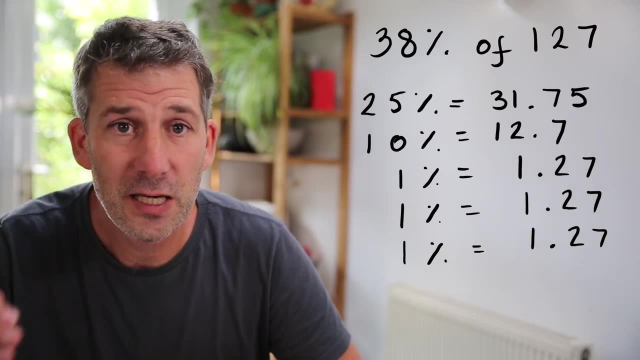 it will take a little bit of time to do these sorts of questions, um, but you can still do them, and you can still do them without a calculator. all you've got to do is add up that list of numbers which, if you've written it down and you've taken a bit of care to make sure your columns are all. 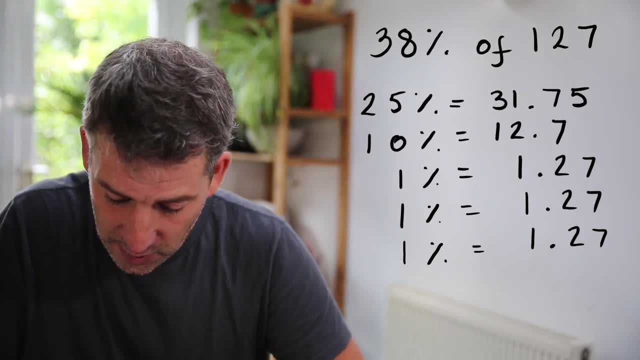 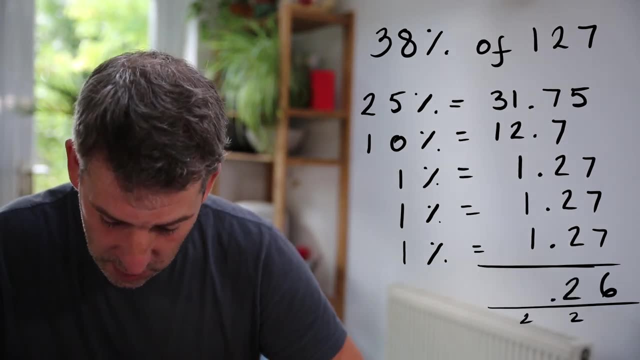 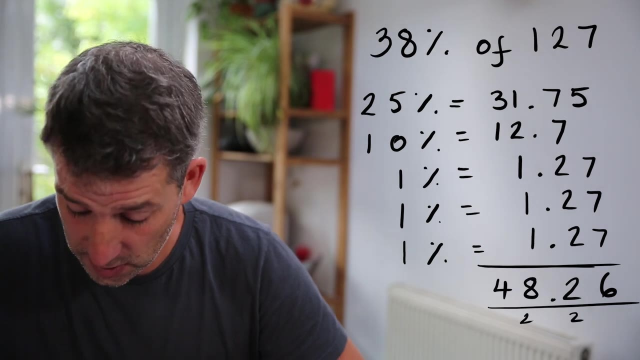 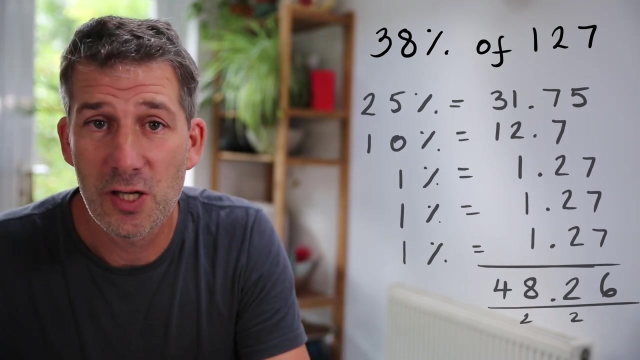 that big a deal. it takes a little bit of time. so if i add these up- so 21, 26, carry the two over um, so i make that 48.26, 48.26 um. i would say if you can do that, you can pretty much do any of them. 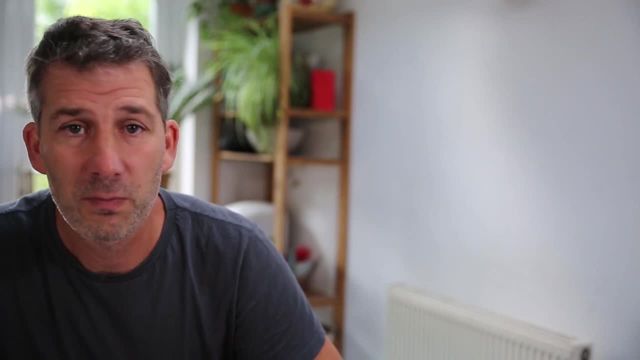 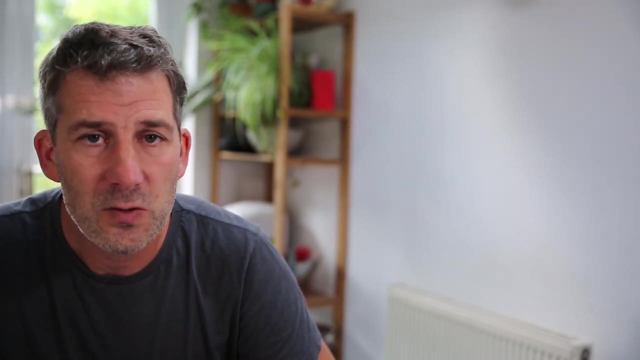 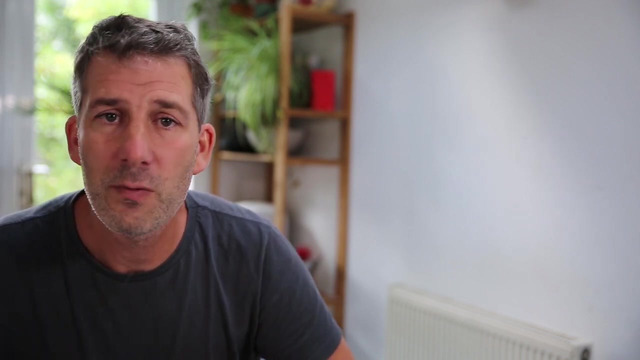 we haven't got into decimals today, how you would find, for example, a three point, one percent or something, and we haven't looked at perhaps some slightly more efficient, more advanced ways of doing the same sorts of things. but we'll get onto that in the second part of the video. um, i would just keep practicing that. um, i'll leave a few questions. 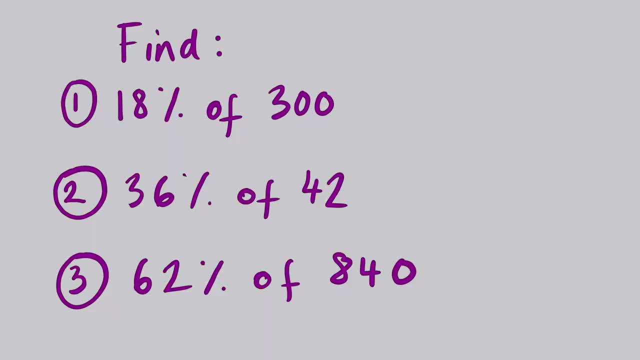 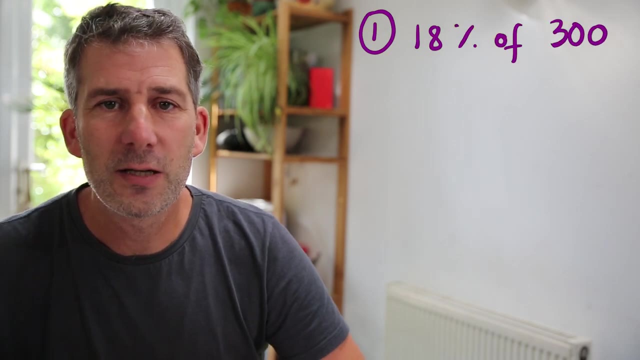 and then i'll, you know, pause the video and i'll put the answers up a few seconds later. okay, here are three questions for you to have a go at. pause the video and i'll give a very brief explanation with some answers in just a moment. so question one, which is to find eighteen percent of 300: the way i did it was, i found ten percent.